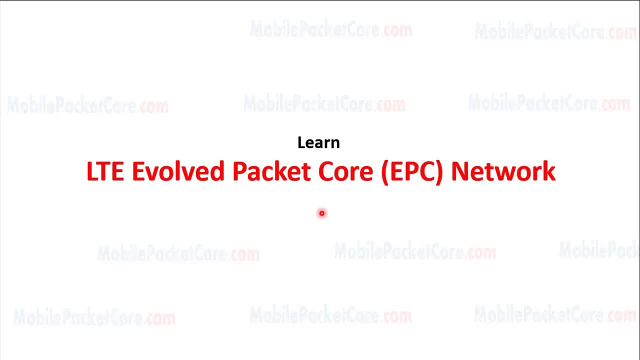 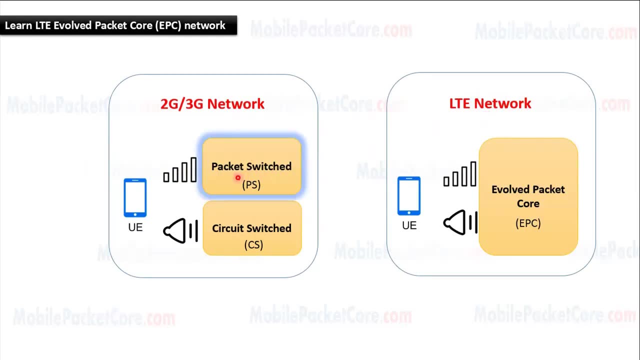 Hello and welcome to this course. Mobile network contains different technologies: 2G-3G network and LTE network. The core network in 2G-3G contains the packet switch domain that handles the data sessions of the users and the circuit switch domain that handles the voice calls of the users. 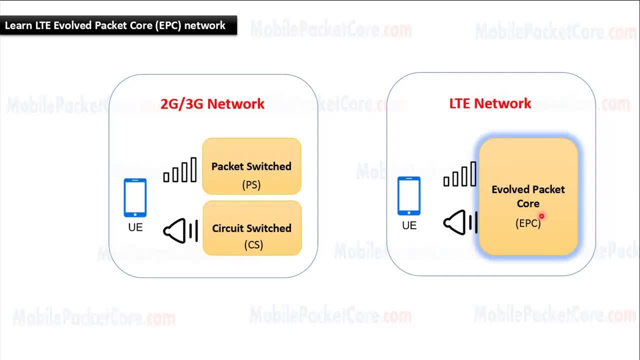 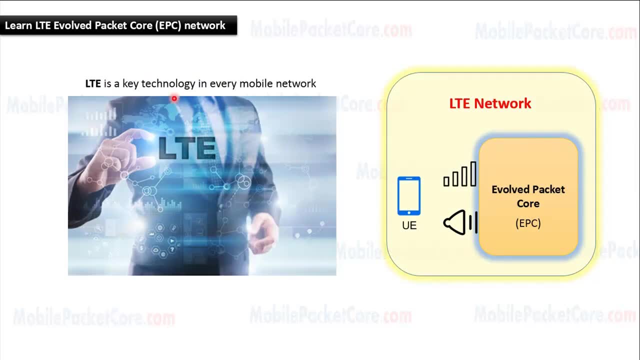 While in LTE, the core network contains only one domain, which is the evolved packet core that handles both the data sessions and the voice calls of the users, LTE is a key technology in every mobile network. Therefore, having a solid knowledge in LTE evolved packet core is essential for every PS core engineer. 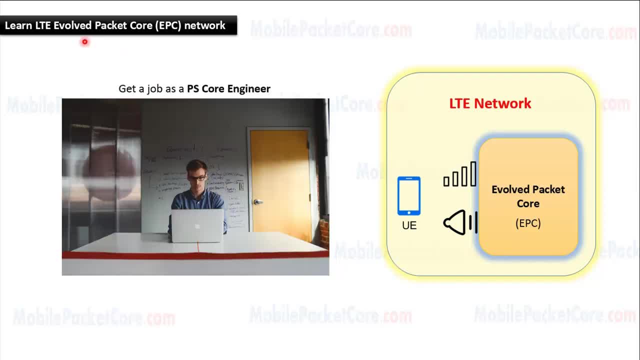 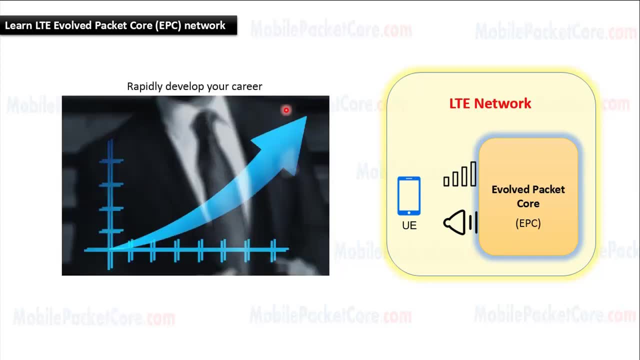 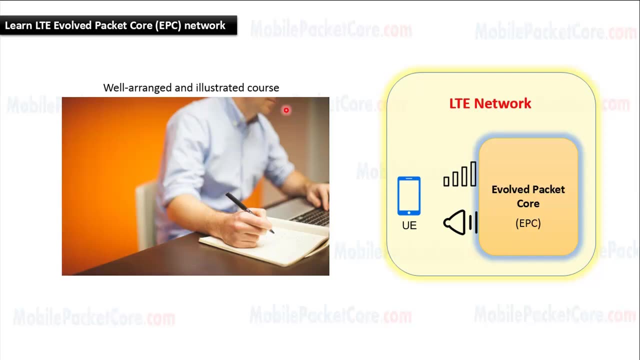 This course illustrates LTE evolved packet core network. This course highly increases your chances to get a job as PS core engineer and helps you to rapidly develop your career after you start your job. This course is well arranged and illustrated and gives you the important topics in a very clear and easy manner. 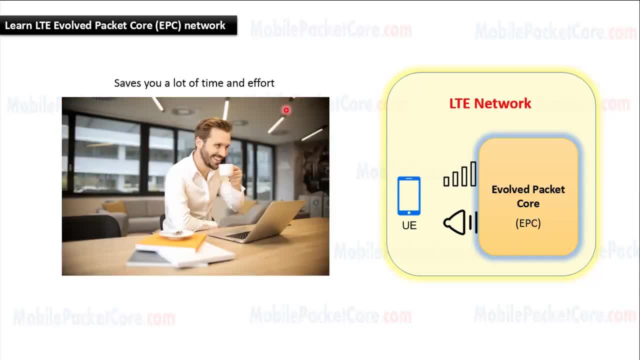 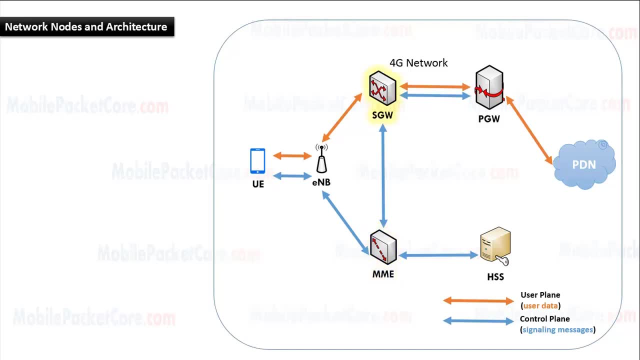 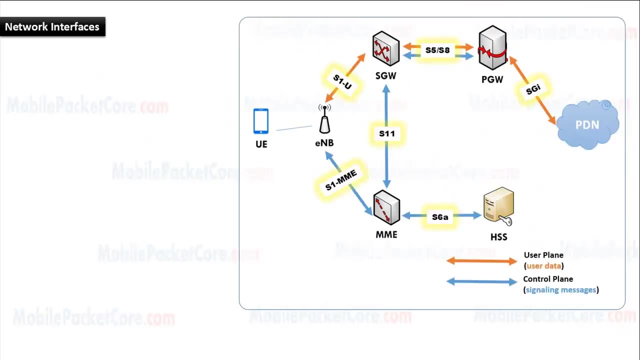 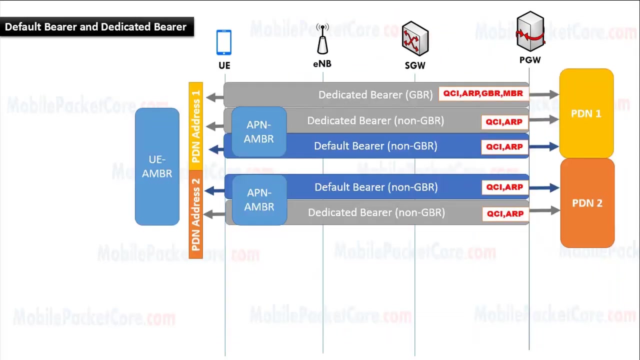 which saves you a lot of time and effort searching. In this course, you will learn network nodes and architecture, including MME, SGW and PGW, HSS, PCRF and OCS, DPI, CG and DNS, in addition to network interfaces and basic procedures including attach and detach, default bearer and dedicated bearer activation. 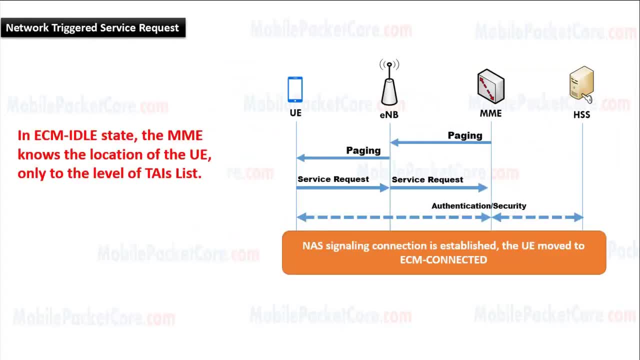 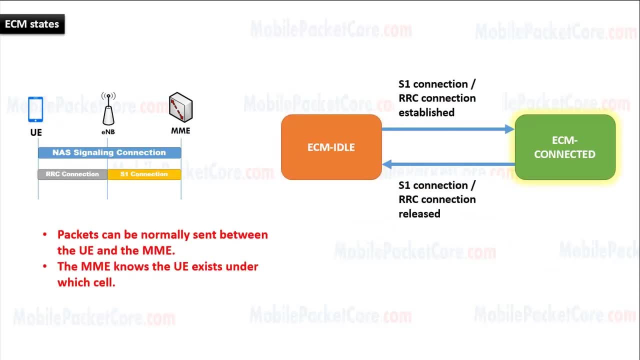 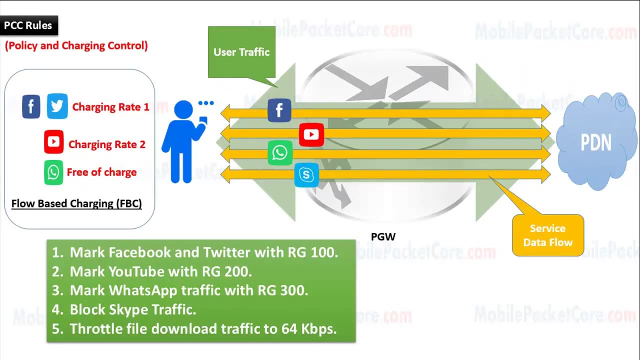 tracking area update handover service request and network triggered service request. different UE states, including EMM registered and EMM deregistered, ECM connected and ECM idle policy and charging control, including online and offline charging, volume time and event based charging, flow based charging and PCC rules. 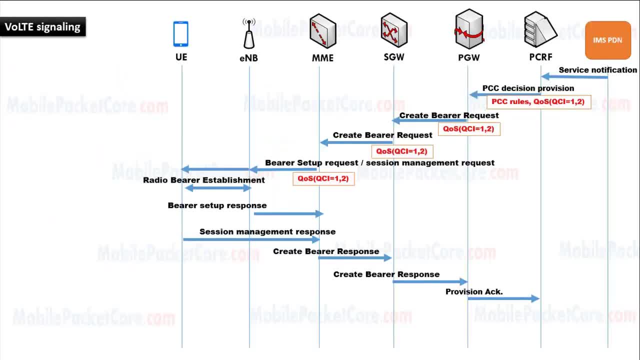 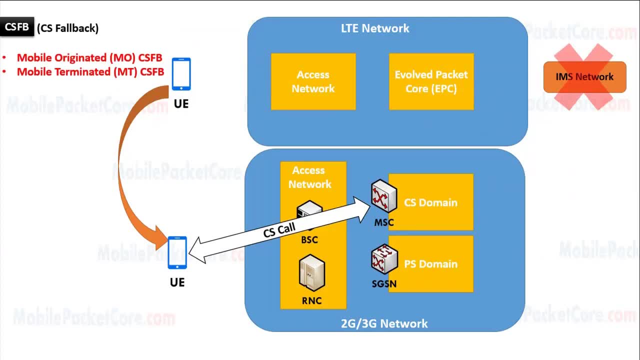 in addition to the fundamentals of voice over LTE, including VoLTE signaling, SRVCC and CS fallback. I hope this course will be great for you. Let's start learning. 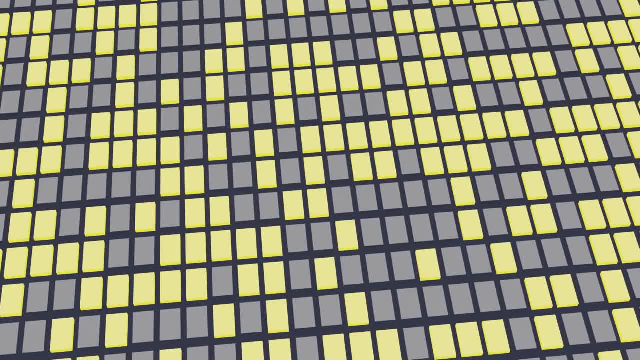 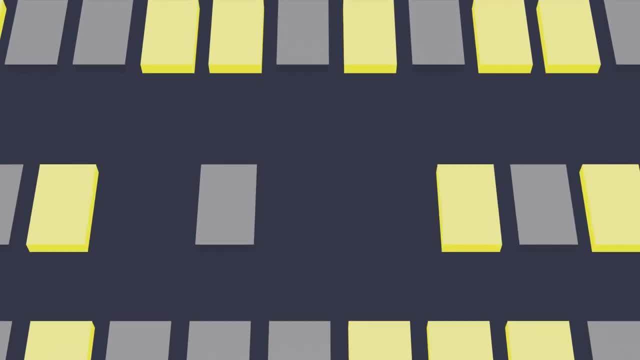 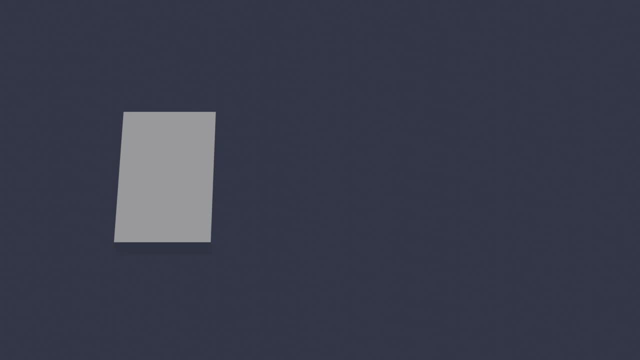 Inside your computer are billions of units called transistors. These transistors serve a variety of purposes, but they commonly act as a sort of very small light switch. Each switch can be turned on or turned off. Computer scientists will often represent a switch that's turned on with the